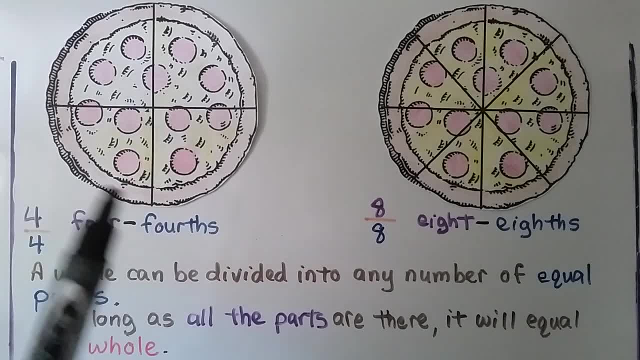 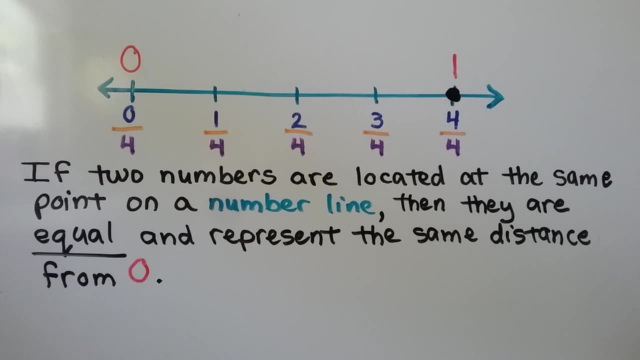 It will equal one whole. We have all 4 parts. nobody's eaten any, so we have 4 fourths and all the parts are here. It's a whole pizza. just like that's a whole pizza. If two numbers are located at the same point on a number line, then they are equal, and 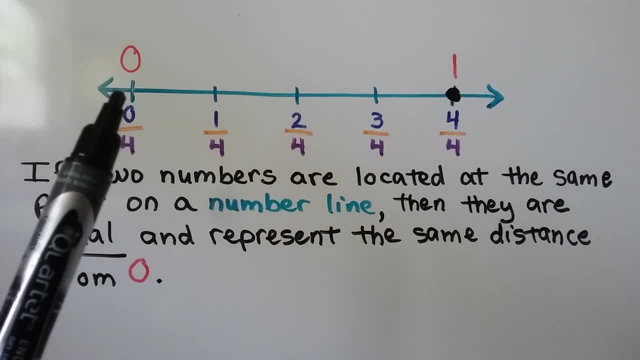 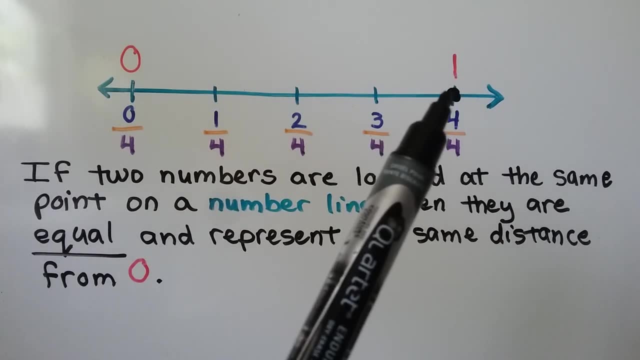 represent the same distance from zero. Here we have zero and we've got 4 fourths, which is also 1.. 4 fourths is at the same point as 1 on the number line, so they represent the same distance from zero and they're equal to each other. We can complete the number. 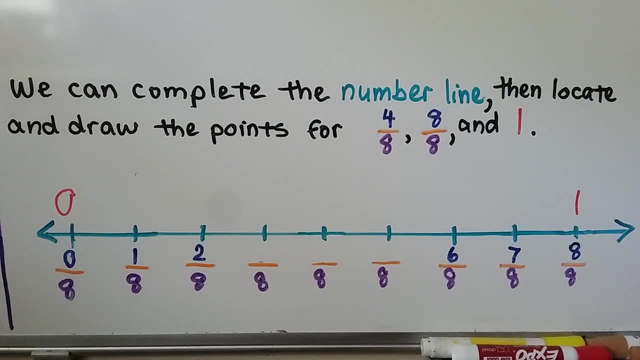 line, then locate and draw the points for 4 eighths, 8 eighths and 1.. So we look at the numbers on the bottom here for the scale and here's zero, that's 0 eighths, and we can. 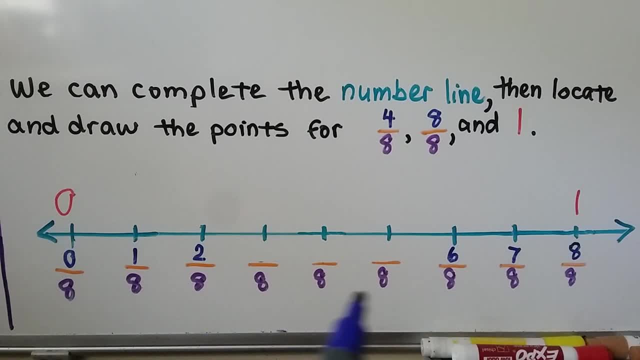 see, it's in eighths because that's what the denominator is. It tells us it's split into 8 equal parts. If we're at 0, we have 0 eighths. We don't have any Here. we're at 1 eighth, 2 eighths and we need to fill in these Do. 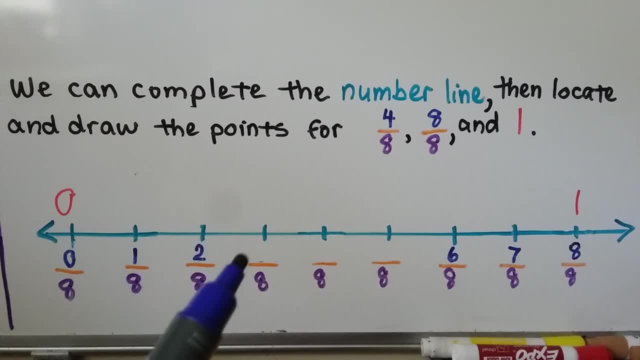 you know what's missing here? It goes 1,, 2,, and then that would be 3 eighths, then we'd have 4 eighths, then 5 eighths, then 6 eighths, 7 eighths and 8 eighths. 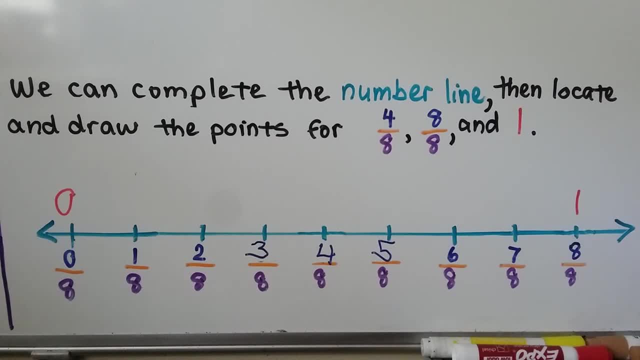 And we can locate and draw the points for 4 eighths- that's right here- and 8 eighths, and 1 is over here. 8 eighths is equal to 1, so we only have 2 points drawn on the line. 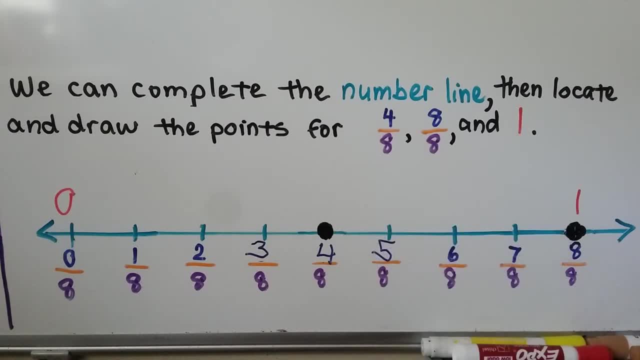 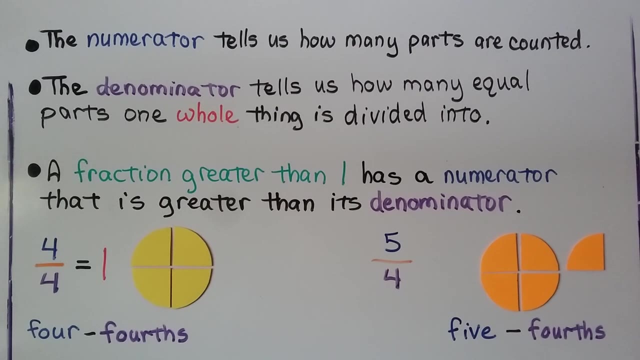 for these 3 numbers because 8, eighths and 1 are the same point. So if 2 numbers are located at the same point on a number line, they're equal and represent the same distance from zero. A numerator tells us how many parts are counted or how many are shaded, and the denominator 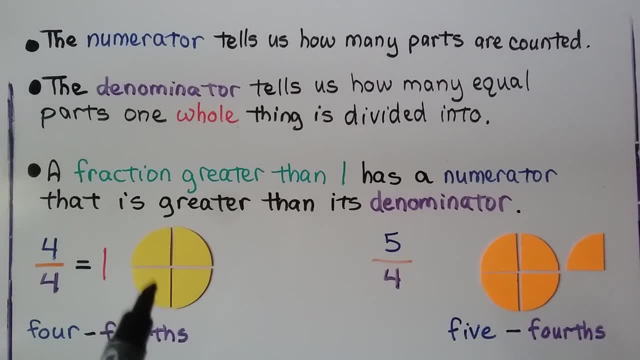 tells us how many equal parts one whole thing is divided into. We have a whole circle and it's in 4 parts. It's divided into 4 parts, so our denominator is a 4.. We have all 4 parts of the 4, so we have 4 fourths. We have one whole circle. 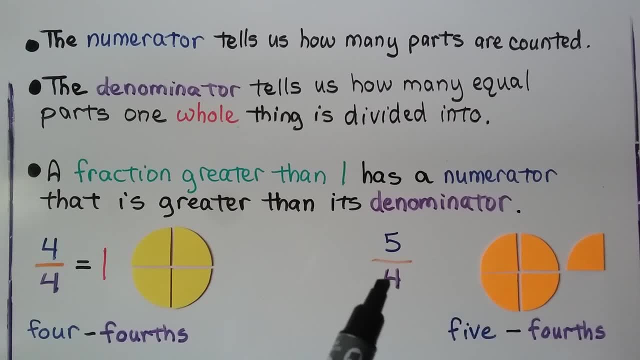 Here it's divided into 4ths and we can see our denominator is a 4, but look, we have 1, 2, 3, 4, 5 parts, that's 5 fourths. Our numerator is larger than our denominator, A fraction. 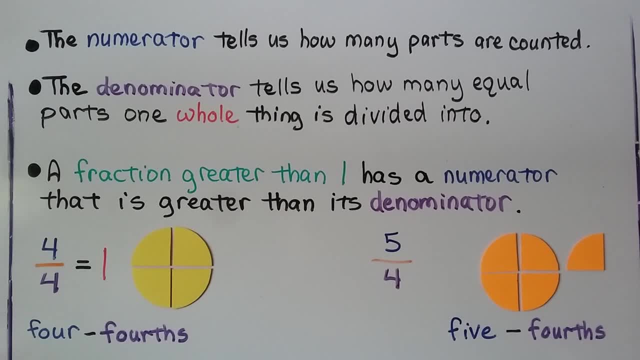 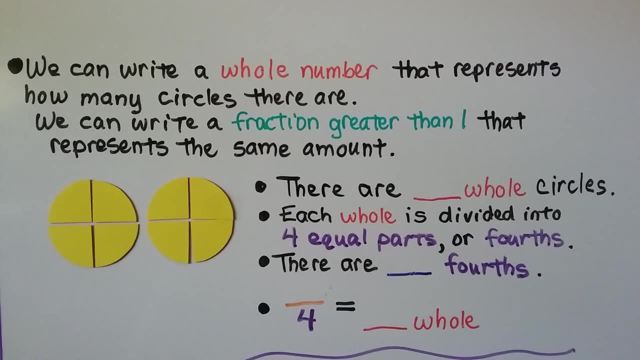 5. fourths, our numerator is larger than our denominator. A fraction greater than 1 has a numerator that is greater than it's denominator. So this is a fraction greater than 1, 5 enter greater than 4.. We can write a whole number that represents how many circles there are. 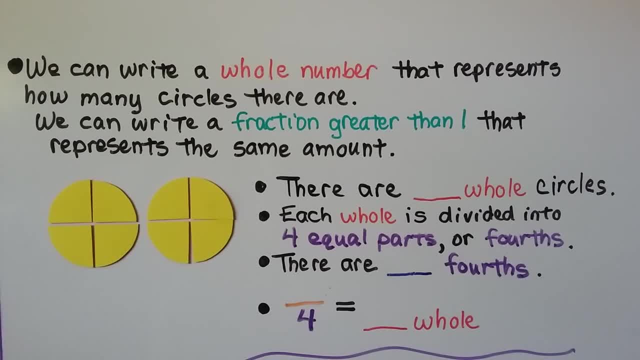 and we can write a fraction greater than one that represents the same amount. Here we have one whole circle and another whole circle, so there are two whole circles. Each whole is divided into four equal parts: one, two, three, four. one, two, three, four. 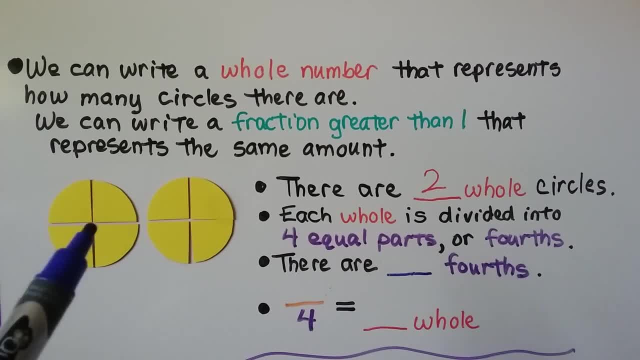 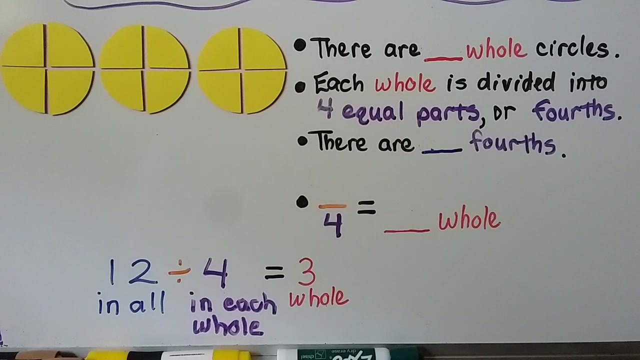 and there are four in each. so we have four, five, six, seven, eight fourths. We have eight fourths. We'd write the fraction like this: Eight fourths is equal to two whole. For this one we have one, two, three whole circles. 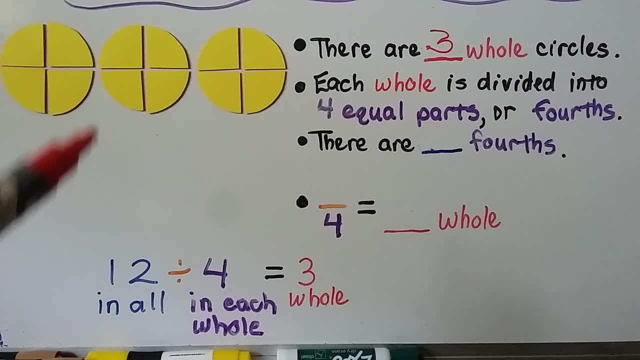 Each whole is divided into four equal parts or fourths, and there are four equal parts: Four, five, six, seven, eight, nine, ten, eleven, twelve, fourths. We write the fraction as twelve fourths. Twelve fourths is equal to one, two, three whole circles. 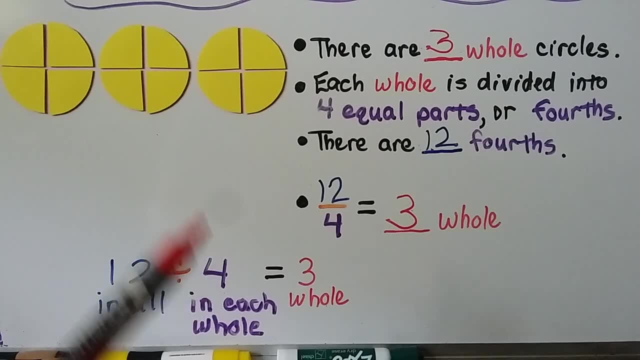 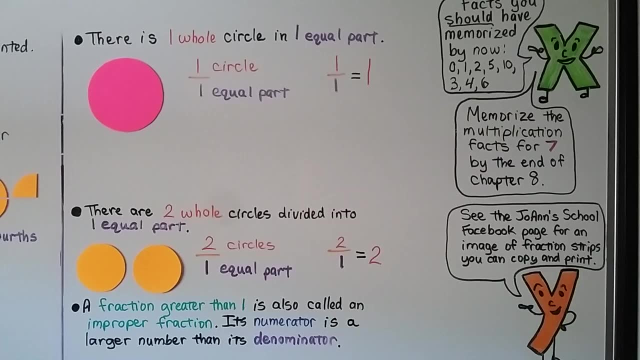 If we have twelve in all and there's four in each whole circle, then we have three whole circles. Here we have this pink circle. It's a whole circle and it's not split up at all, is it? It's just one whole, equal part. Our numerator would be one, Our denominator would be one. 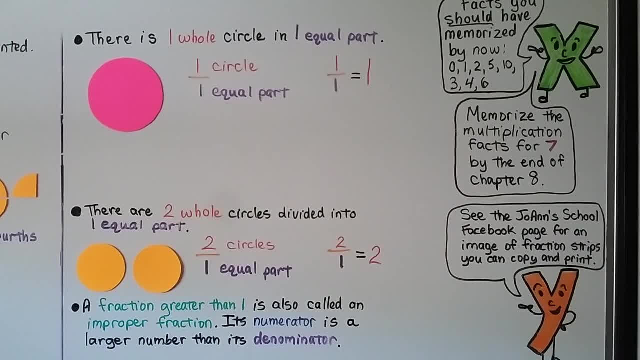 We have the same numerator and denominator, The whole thing is equal to one whole. Now we have two whole circles divided into one equal part. There's one whole part. here We have two circles that each have one equal part. Our numerator is a two. Our denominator is a one. It's equal to two whole. 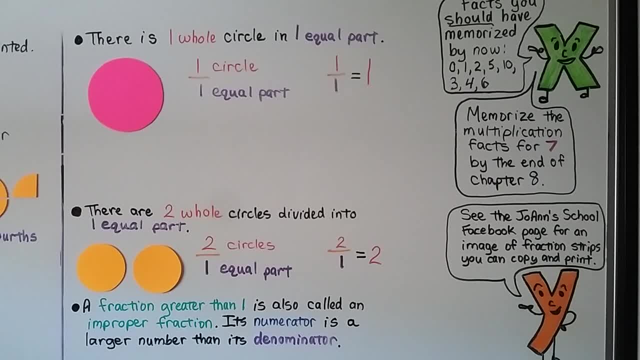 A fraction greater than one is also called an improper fraction. You're going to hear it called that in middle school. Its numerator is a larger number than its denominator, And keep in mind that I have an image of fraction bars on my Facebook page in the image section that you could copy. 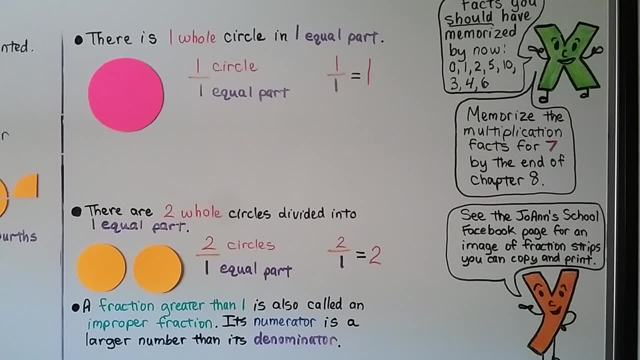 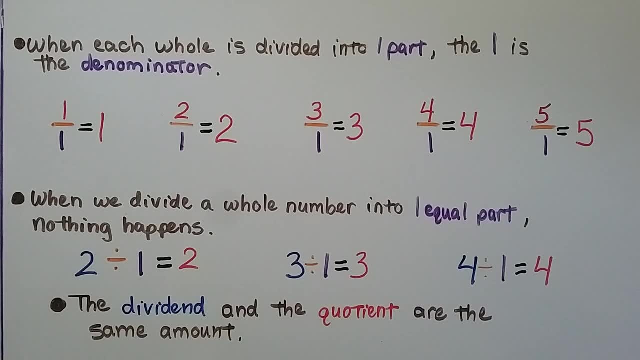 paste and print. if you want to use some fraction bars, I'm using my Facebook page to copy and paste the bars. use some fraction bars for your homework. When each whole number is divided into one part, the one is the denominator. So if we have one circle, that's in one part, we have one. 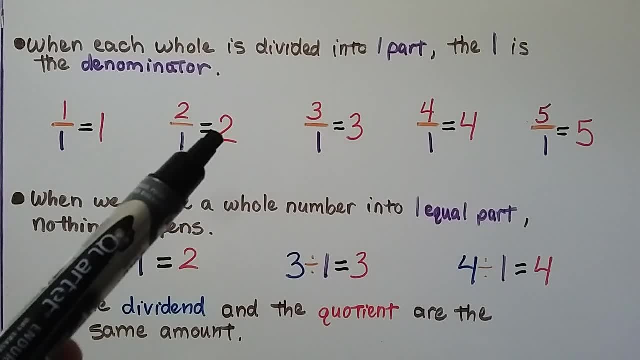 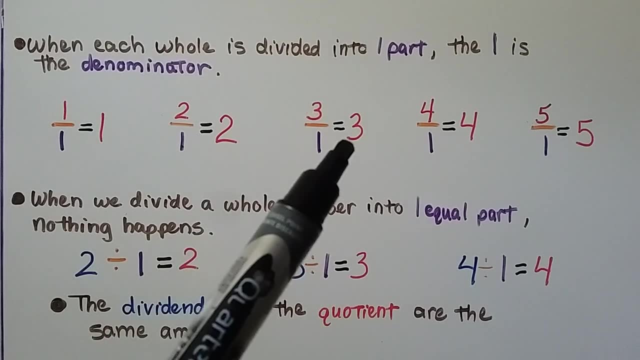 If we have two circles that have one part, we have two whole. If we have a three as the numerator and a one as the denominator, we have three whole. Four as the numerator with one as the denominator, we have four whole, And here we have five whole. 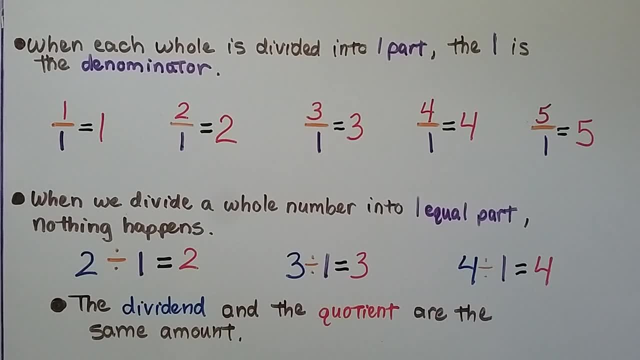 When we divide a whole number into one equal part, nothing happens. It stays the same. The dividend and the quotient are the same amount. Two divided by one is equal to two. Three divided by one is equal to three. Four divided by one is equal to four. 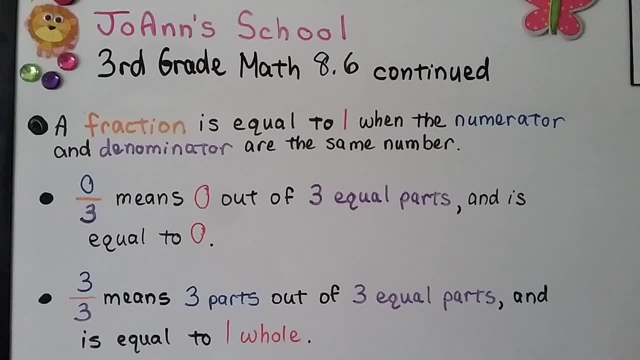 A fraction is equal to one when the numerator and denominator are the same. If we have zero thirds, it means we have zero out of three equal parts, and that's equal to zero. We split a candy bar into three parts, but we didn't eat any. 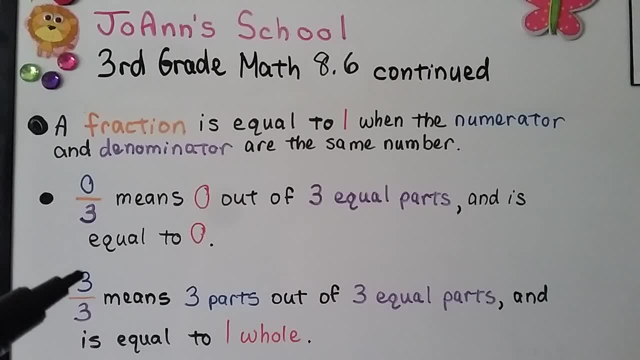 So we ate zero candy bar When we have the same numerator and denominator. three thirds means three parts out of three equal parts and that's equal to one whole If we split a candy bar into three equal parts and we ate all three parts. 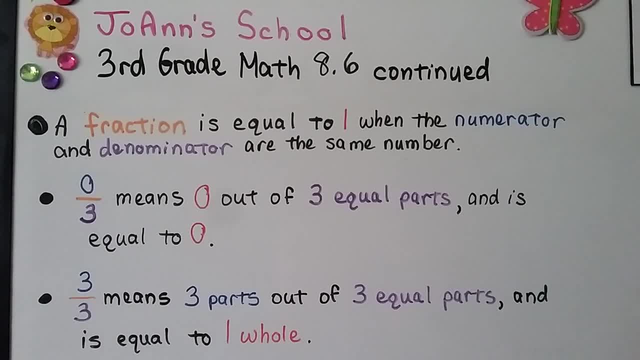 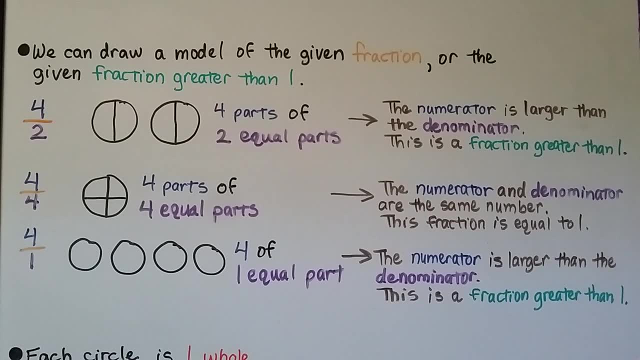 We ate the whole candy bar, didn't we? We can draw a model of the given fraction or the given fraction greater than one. Here we have four halves. It's telling us that a whole thing is split into two parts, but we have four of them. 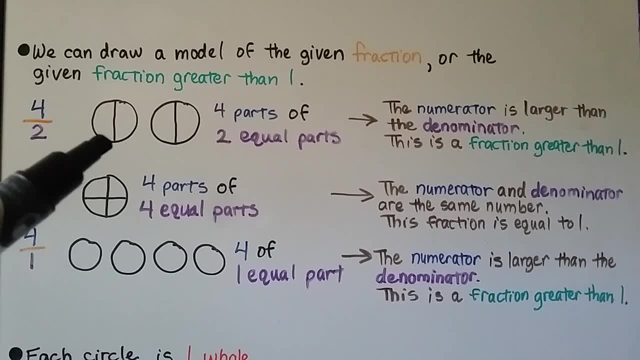 So here we have a whole circle split into two parts, but to have four of them we would have to draw another circle with two parts, wouldn't we? The numerator is larger than the denominator, So this is a fraction greater than one. 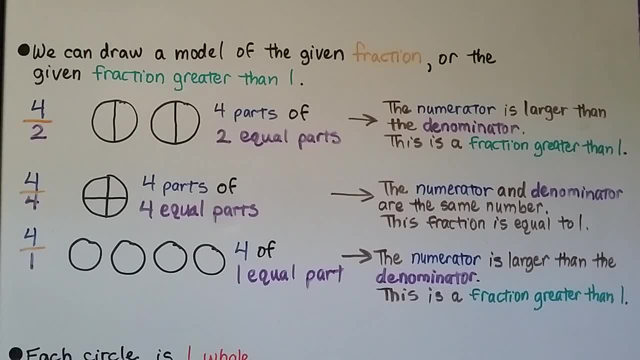 We have four parts of two equal parts. Here we have four fourths, and that means we have a whole thing split into four parts and we have all four parts. The numerator and denominator are the same number, so this fraction is equal to one whole. 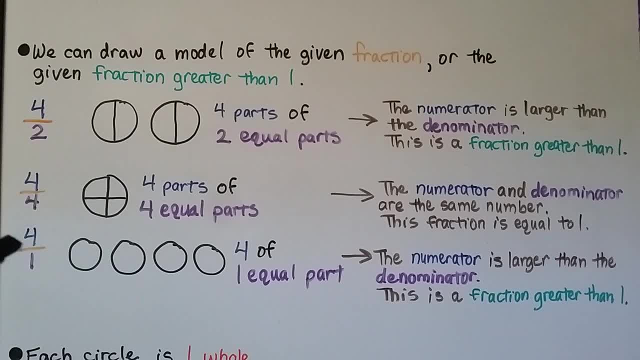 We just have one circle split into four parts. Now we have a numerator that's a four and a denominator that's a one. This numerator is larger than the denominator, So this is a fraction greater than one, and it's telling us that a whole thing is just. 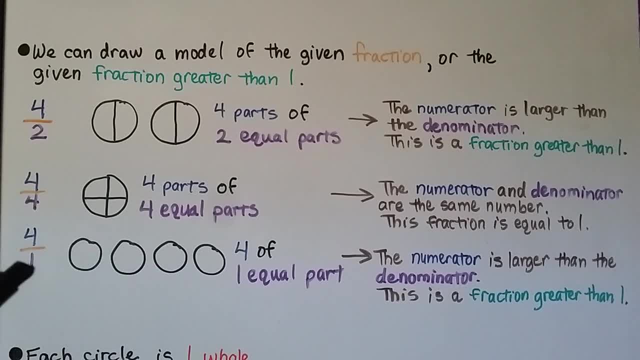 in one part, but we have four of them. So if we have a whole thing, that's one part like this, it's got no cuts to it, no lines in it, but we have four of them. So we have four of one equal part. 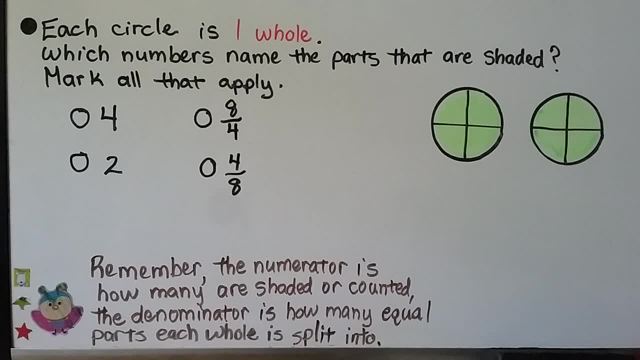 Take a look at these green circles. Each circle is one whole circle. So which of these numbers name the part of the denominator? I don't know, I don't know, I just don't know, I don't know, I just don't know. 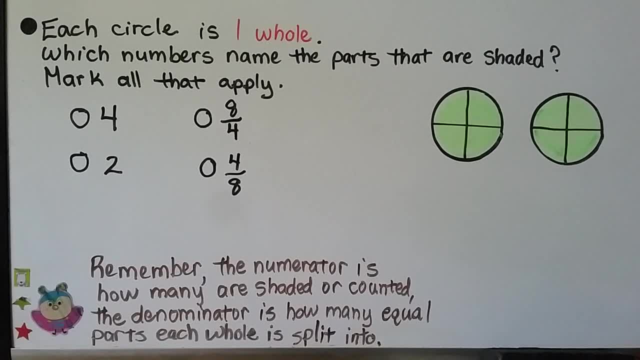 Okay, So we have four equal parts that are shaded. We need to mark all that apply, So remember: the numerator is how many are shaded or counted, and it looks like in both circles they're all shaded, aren't they? And the denominator, the bottom number, is how many equal parts each whole is split into. 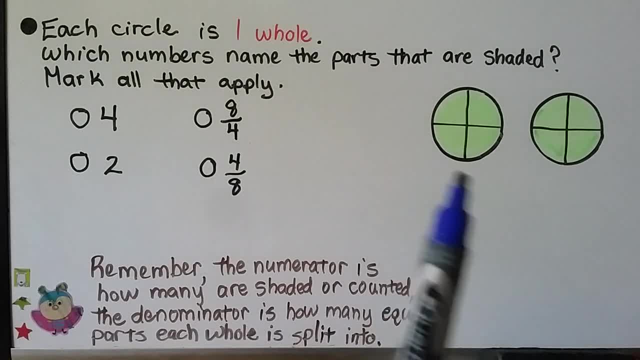 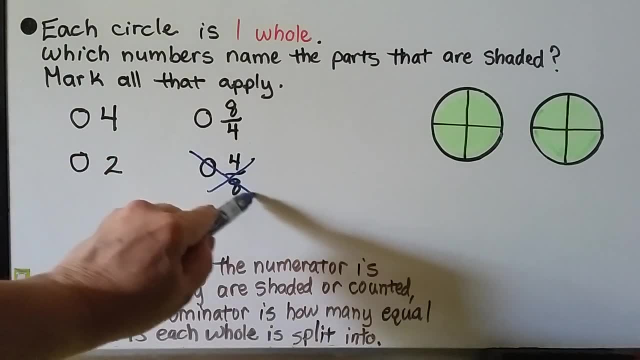 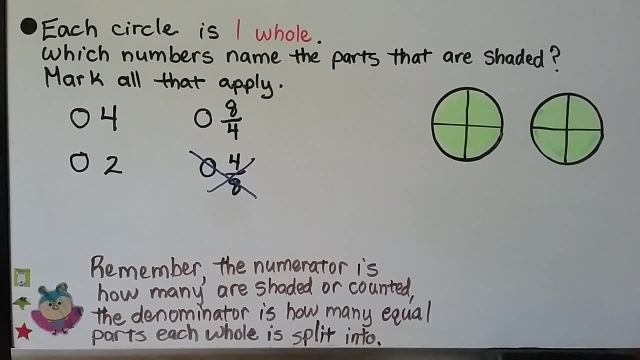 We take a look at this whole circle, it's split into four parts, So is this one. So we know our denominator must be a four, So it can't be this one because that denominator's an eight, isn't it? We count how many parts are shaded. We have 4,, 5,, 6,, 7, 8.. 8 parts are shaded and 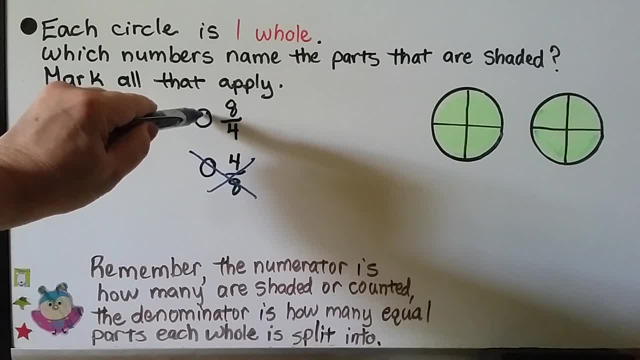 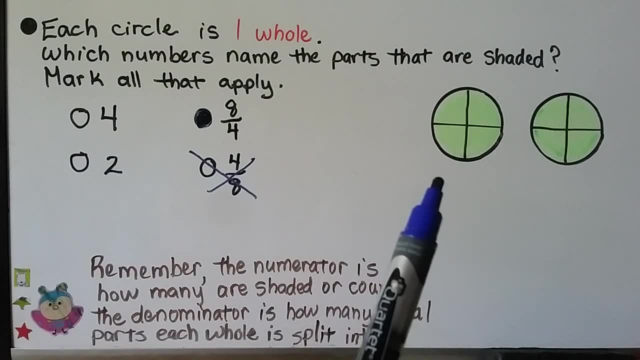 we know the denominator is supposed to be a 4, so we know this is one of the correct answers that apply. We can also see from the picture that we have two whole circles, so the number 2 for 2 whole also applies. So remember you pick. 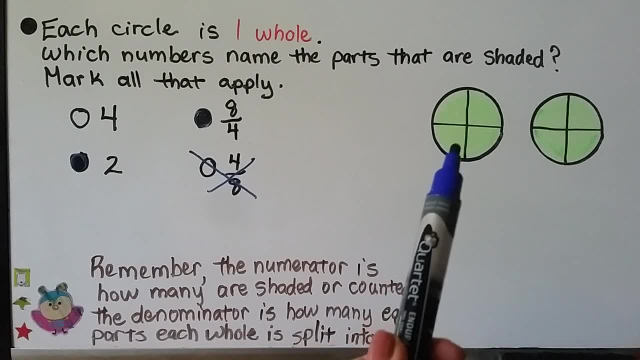 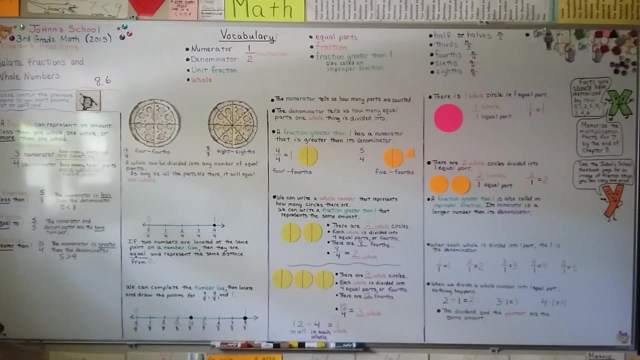 one whole object. you count how many it's split into and that's the denominator. okay, And it's just for one of the whole objects. We're going to talk about fractions of a group next in lesson 8.7, and keep trying. I'm really. 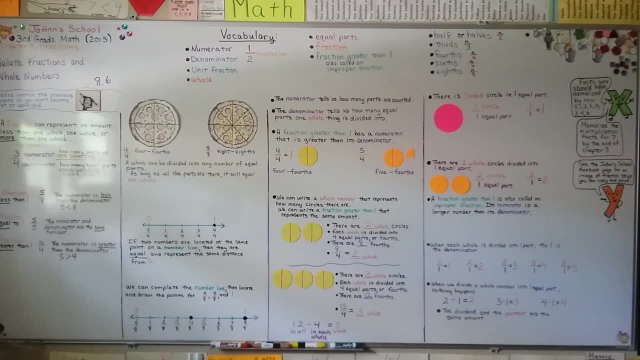 proud of you for watching math videos on YouTube. That's a really good thing and, gosh, I'm so proud of you. I hope you have a really good day and I'll see you next time. Bye. 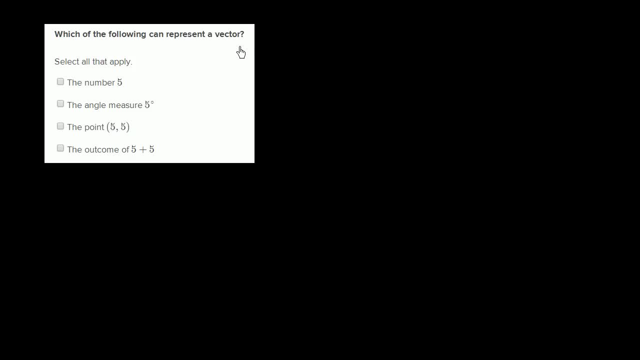 Which of the following can represent a vector? So a vector is something that has both a magnitude and a direction. So let's see which of these could represent something that has a magnitude and a direction. So the first choice right over here is the number 5.. 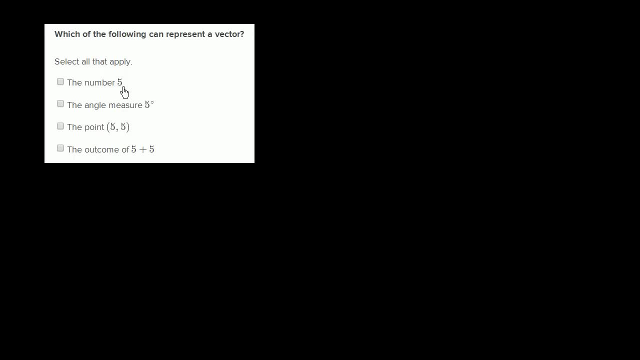 Well, 5 could represent a magnitude. You could say essentially how large something is, but that's all the information has. It doesn't say 5 in a certain direction. So this one by itself would not be a or it couldn't represent a vector. 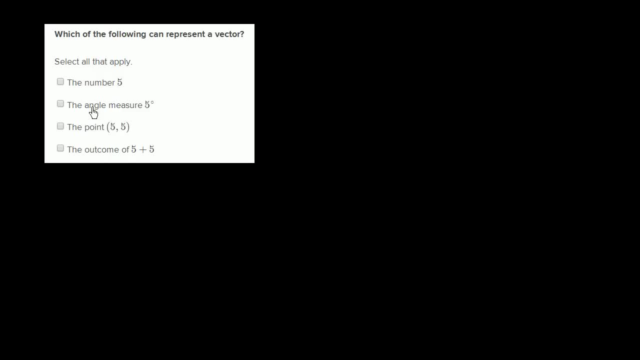 You would need to specify a direction as well. The angle measure 5 degrees. Well, the angle measure 5 degrees could represent a direction. If you say it's 5 degrees, let's say that's the positive x-axis, that's the positive y-axis.